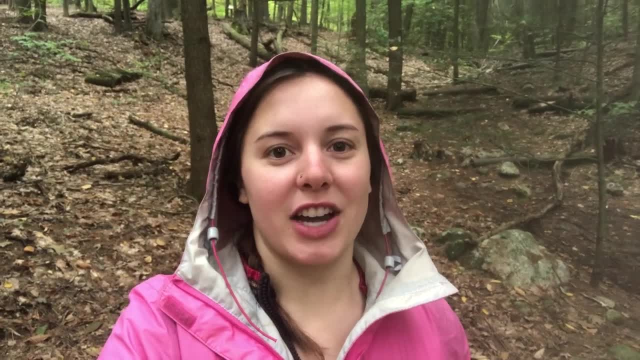 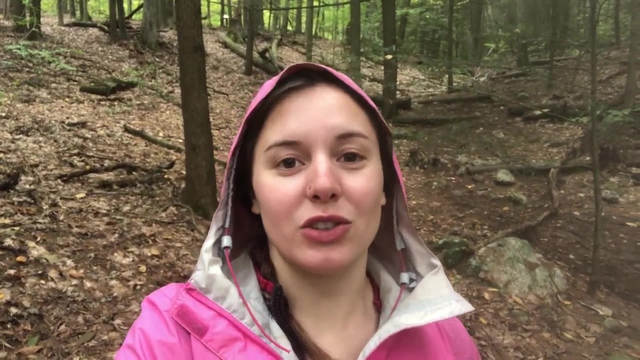 do in the rain outside. So a lot of times many different organisms come out only in this type of weather and I'm going to show you those organisms and some things you can do outside in the rain. So right now it is sprinkling, but it's been pouring the last couple of days. It's 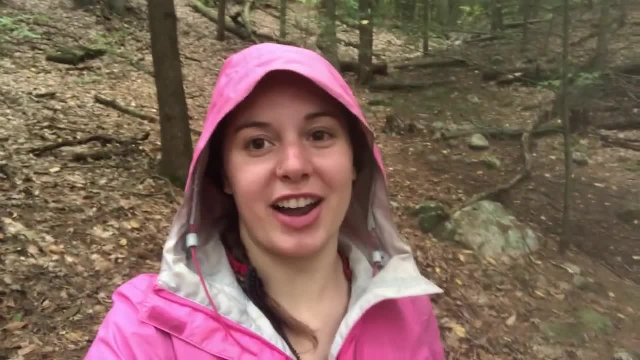 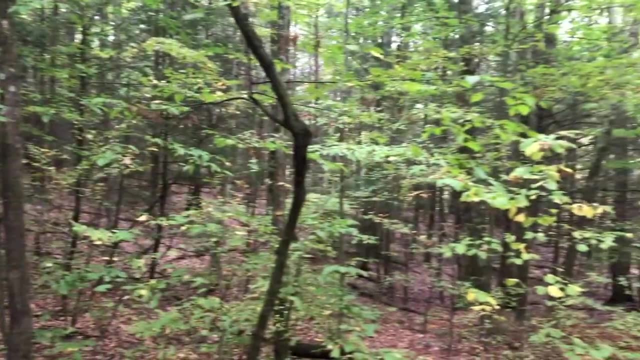 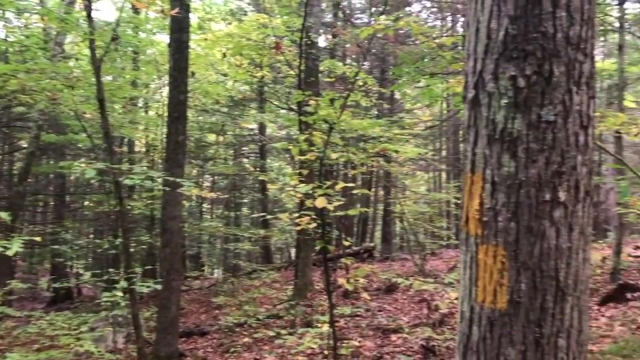 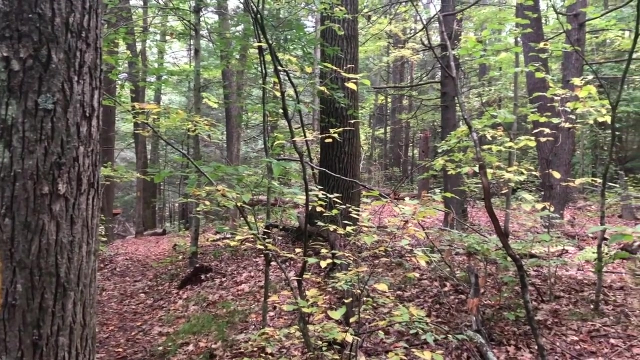 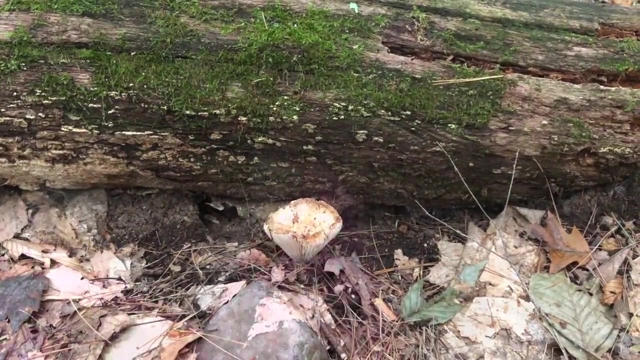 a chilly fall day. I've got my raincoat on, I've got some boots. on the trails are muddy. I'm ready to explore and find some animals. So let's go, let's see what we can find. So right off the bat, I've noticed that there are a ton of new fungus popping out of the ground. 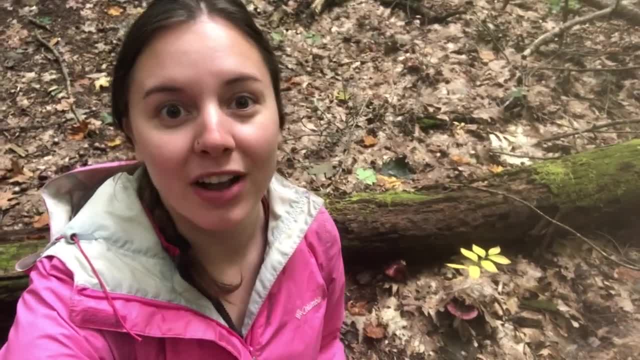 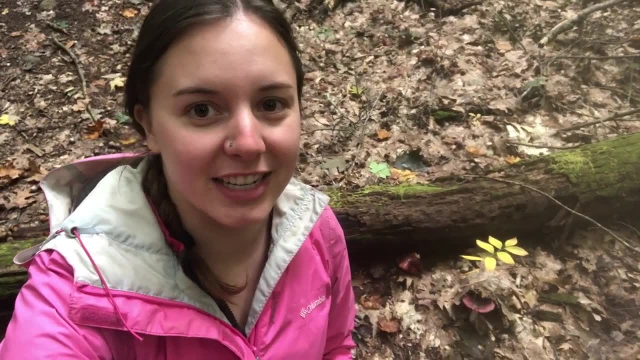 popping out of trees, and that's because a lot of mushrooms thrive on moist, wet conditions. So just on my walk I'm finding a lot of different mushrooms, a lot of different fungus, and it's really awesome, especially this one right here. You can just see it popping out. 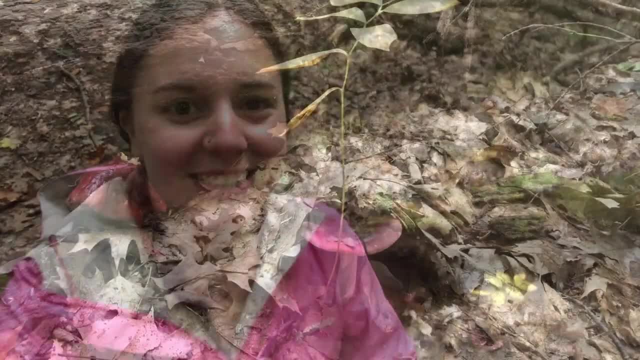 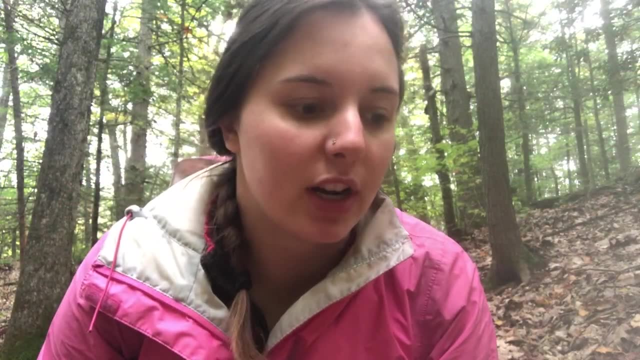 of the leaves. It's super cool to find these. Let's see what else we can find. So I just want to point something out: that if you are looking at fungus in the woods, you don't have to be an expert. You don't have to be hunting for wild edible mushrooms. 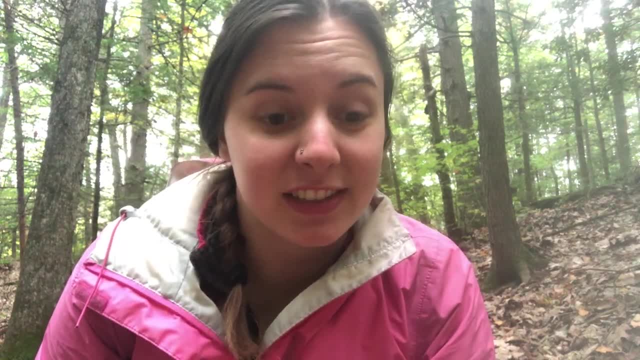 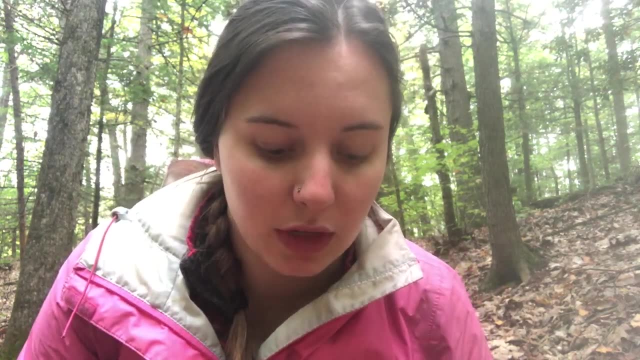 You don't have to know anything about mushrooms. All you need is a sense of curiosity and a willingness to learn. So I just want to get some myths out of the way. You can totally touch any mushroom that you find Touching it. 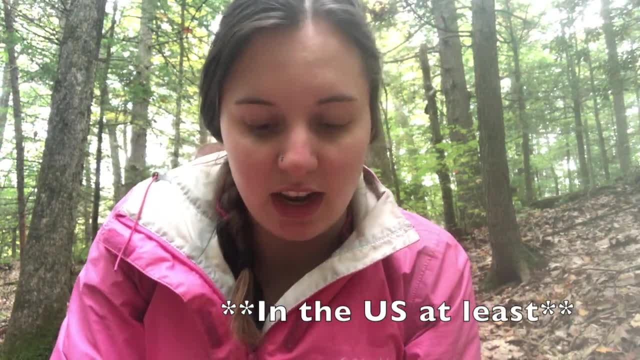 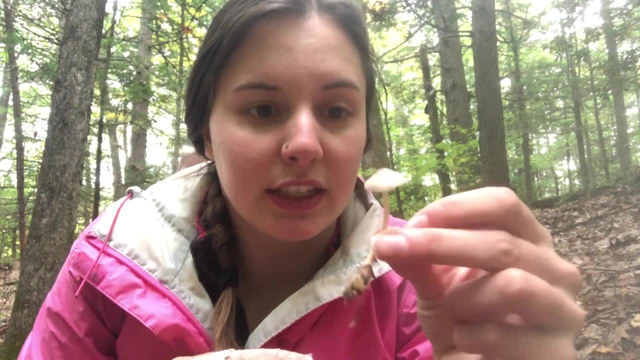 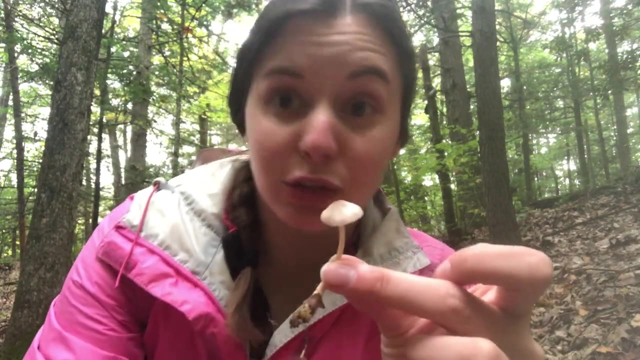 the toxins, if it is poisonous, will not absorb into your skin. And there's many ways to look at mushrooms. So if you don't know anything about mushrooms, this is a good example of a very common mushroom. This is a gilled mushroom. I don't know the official term because I'm not an expert either. 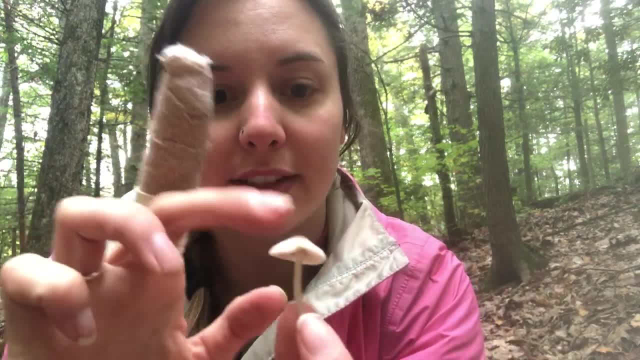 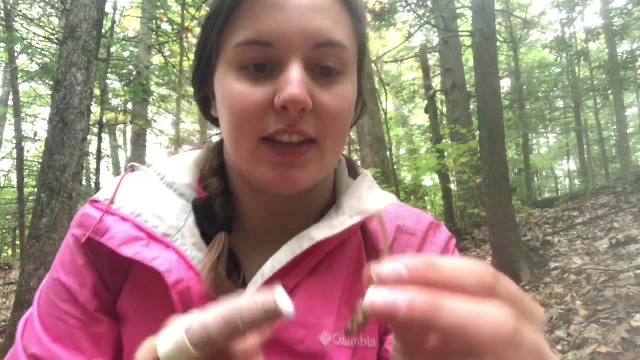 But this is a gilled mushroom and I know that because underneath the cap- this is the cap- there are gills. Let me see if I can show. So there are gills underneath this cap, And so the shape of this mushroom is very classic. You have a stem, or sometimes called a stalk. 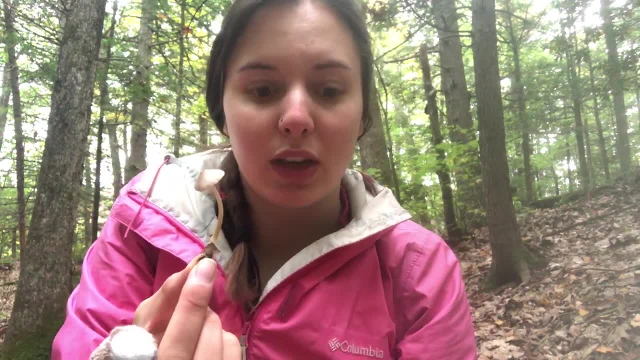 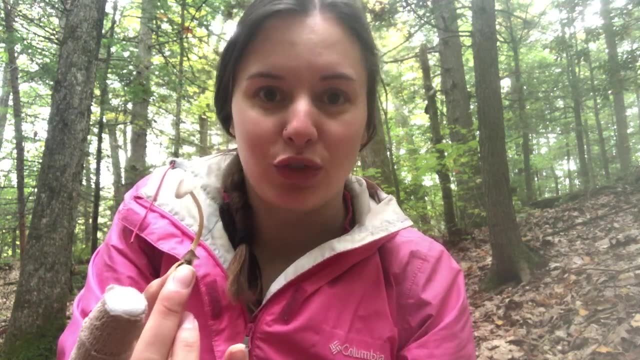 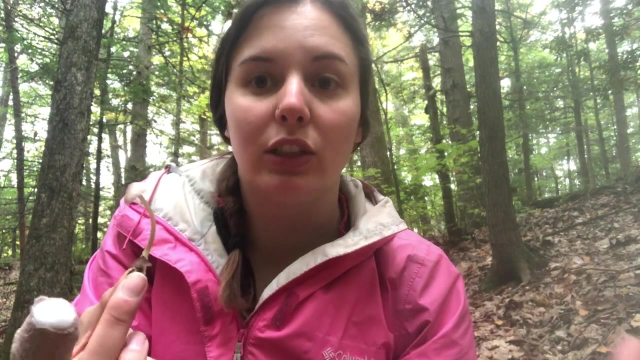 and you have your cap, And mushrooms grow from this giant system of kind of like roots called underground, sometimes inside trees and wood, And so mushrooms are just the fruiting body of this more larger organism that we even know of. So if you are digging in the ground and you see this, 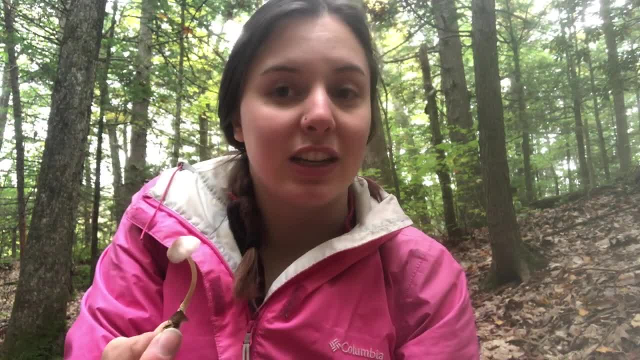 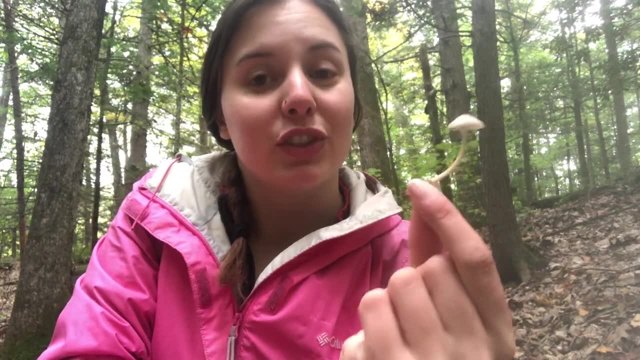 white kind of looks like a spider web. that's most likely going to be mycelium of a mushroom or fungus that hasn't fruited yet. So mushrooms are just the fruiting body of a fungus, And so if you're just a beginner looking at mushrooms, you're going to find a lot of mushrooms that are 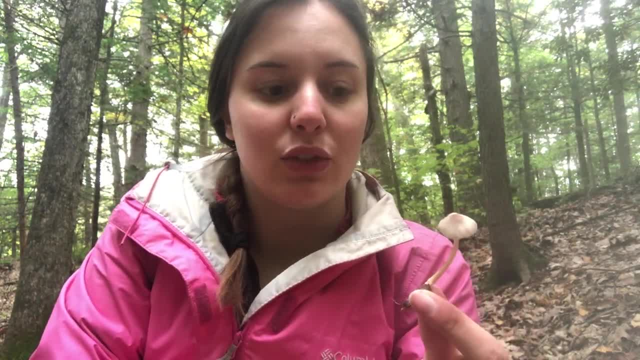 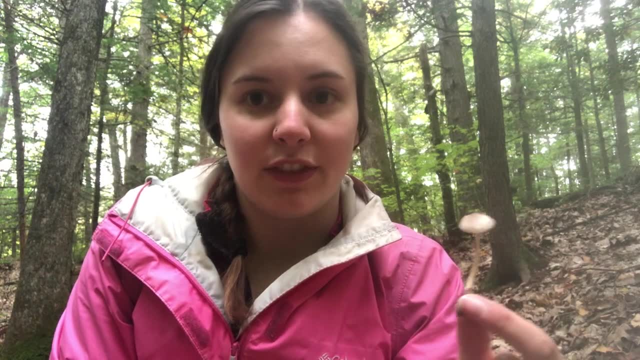 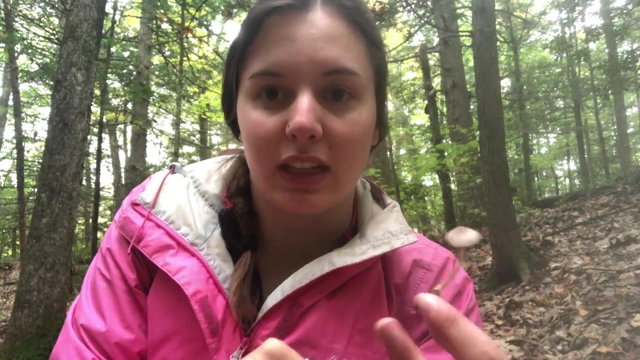 fruiting fungus. One great way to learn about it is to try to record everything you find. So what I like to do? any new fungus that I find, I try to identify its basic characteristics. Does it have gills? Does it have pores? Does it have tooth gills? Is it not a uniform in shape? 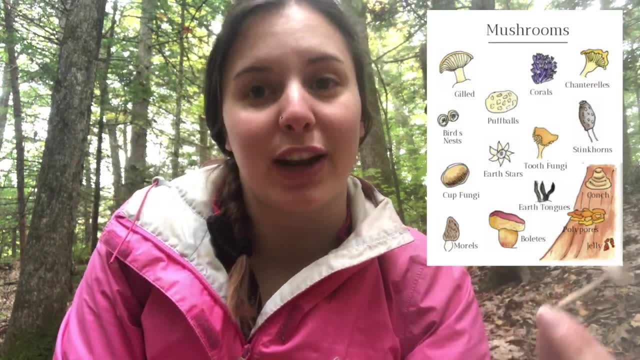 There's a mushroom poster that I actually have in my shop that I will link below so that you can check it out, because it breaks down 15 different types of mushrooms. So if you're a beginner looking at mushrooms, you're going to find a lot of. 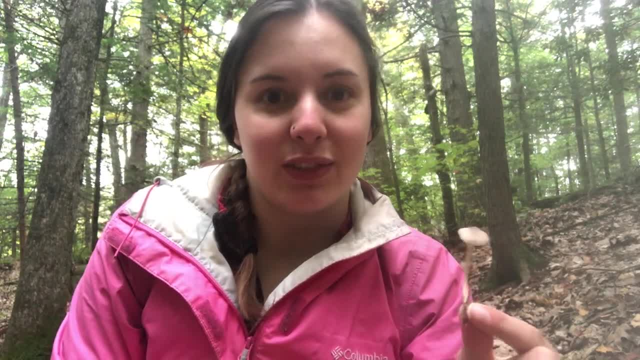 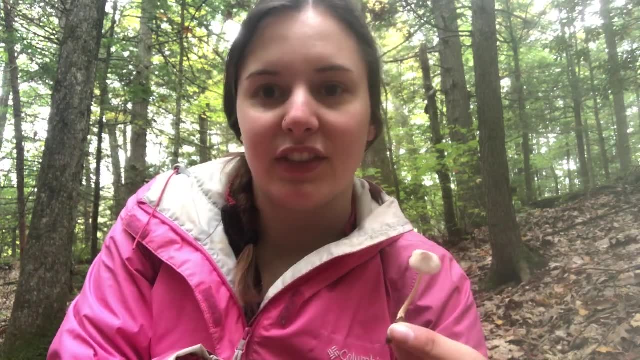 different types of mushrooms, different classifications. That's a great thing to look at. if you're just a beginner, If you can identify if it's gilled or poured or if it is not uniform in shape, then you can. I would take a picture of it And then, when you 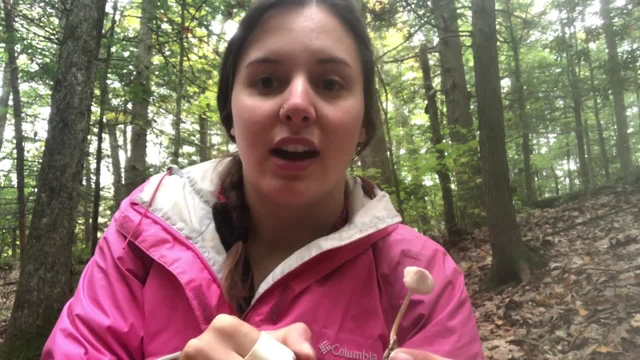 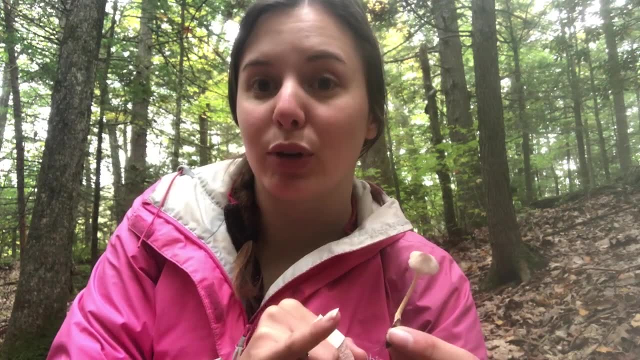 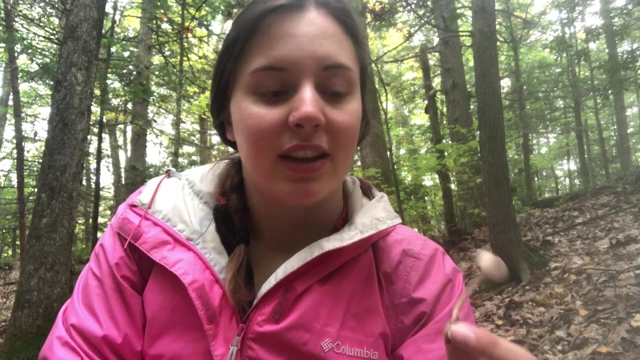 get home, or if you have a field guide, bring it with you. try to identify it in the field or once you get home. Sometimes very hard to identify mushrooms without taking a spore print, which is another thing you can do. You can start to understand what different types of mushrooms are, So that's a great 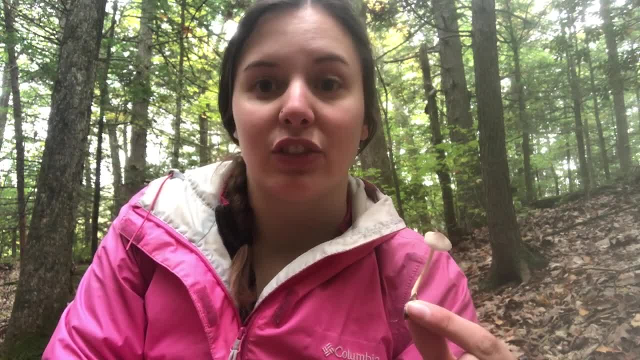 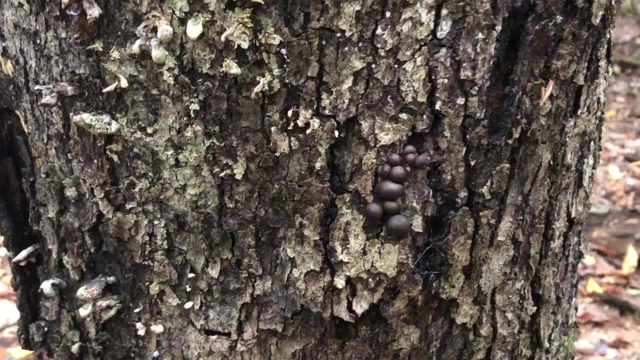 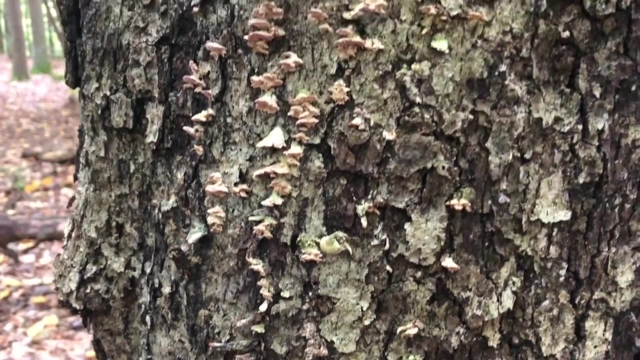 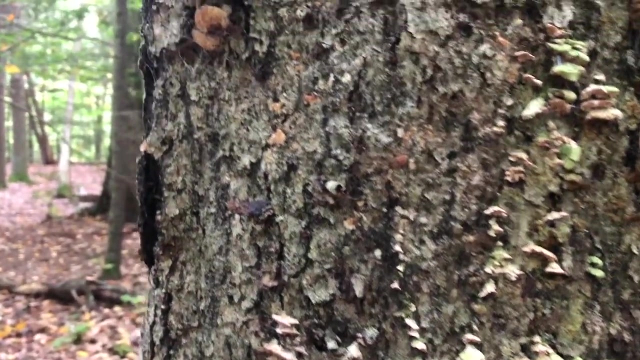 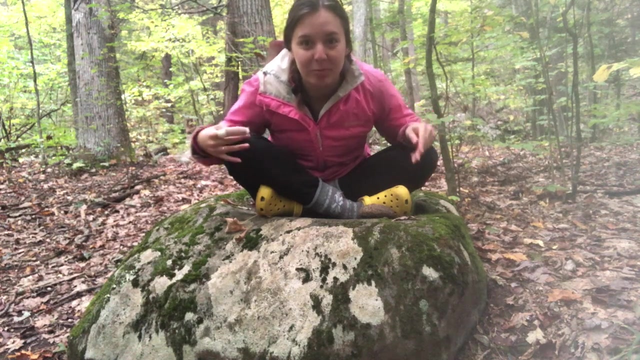 thing you can do on a rainy day is just take some pictures of fungus that's popping up in the ground on trees and try to learn more about it. You don't have to be eating them to learn about them, So another great thing you can do is just simply sit and listen to the sounds around you When it's 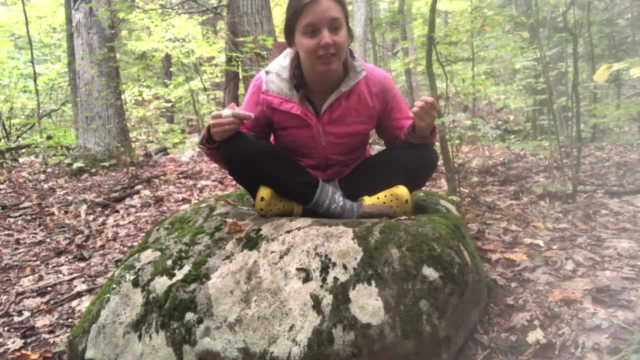 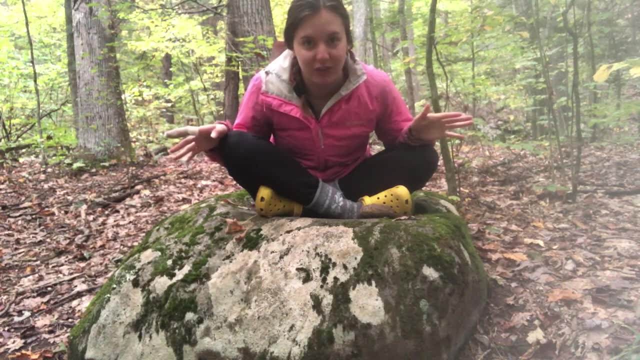 raining out. the rain falling on the leaves and sticks and acorns falling off the trees because of the rain, It creates this beautiful symphony all around you and there's different animals running around, different birds, So just simply sitting, kind of like a meditation, just counting all the different sounds. you 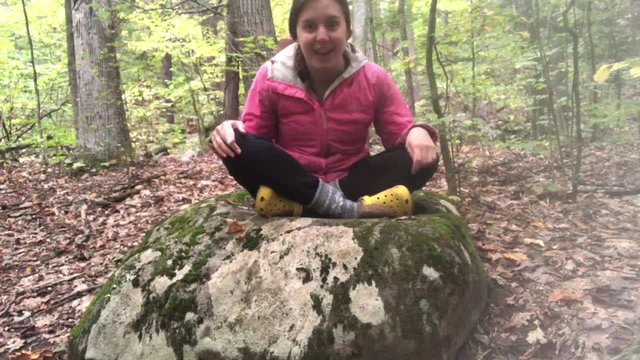 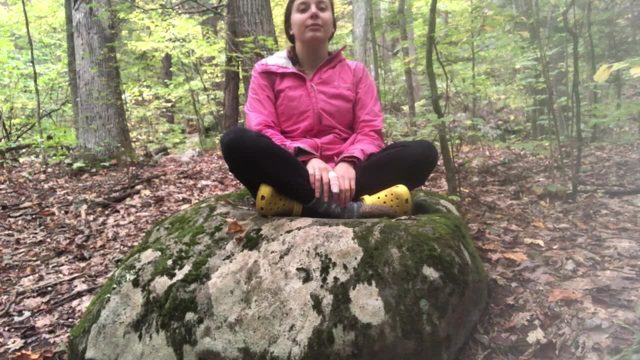 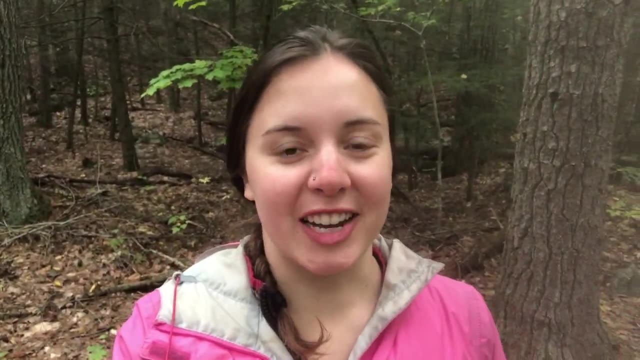 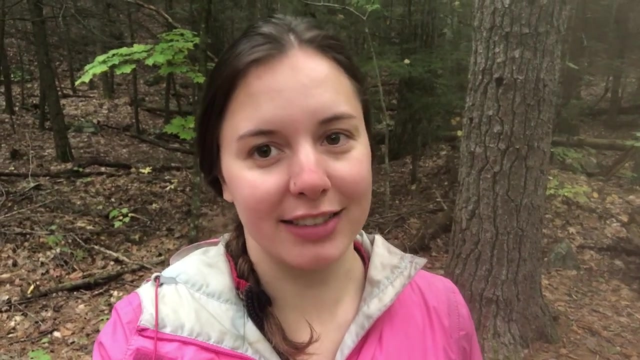 you can hear is a super relaxing thing you can do on a rainy day. Another great thing you can do on a rainy day is look for signs of animals. So, like I said before, the trails are all very muddy. there might be some animal tracks that you can find. I haven't found any animal tracks yet, but I did stumble. 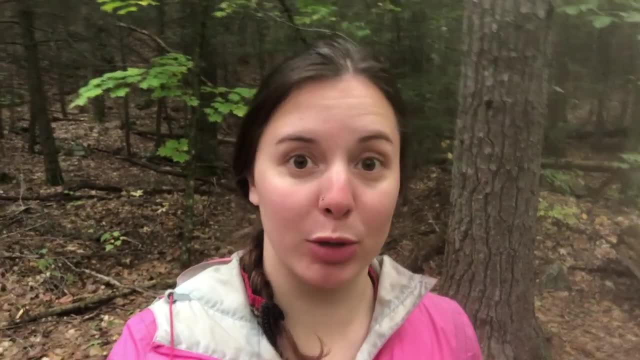 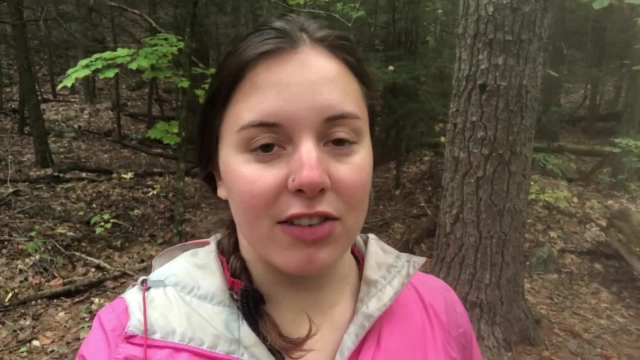 across this log that has a ton of holes pecked from woodpeckers. So woodpeckers peck at the bark of a tree and they eat the insects within the tree, And oftentimes you'll find this on dead trees and trees that have fallen over on. 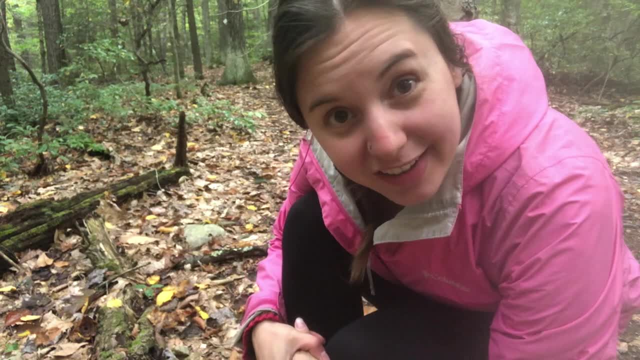 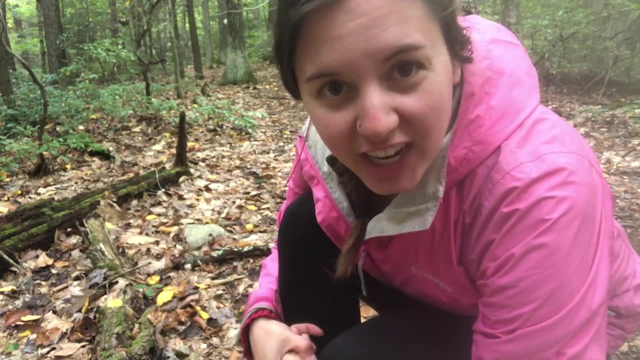 the ground. Another great thing you can do is flip logs and rocks and look for amphibians like salamanders. So I found this really rotted log and I'm gonna see what's underneath it. So whenever you pull up a log or a rock you want to make, 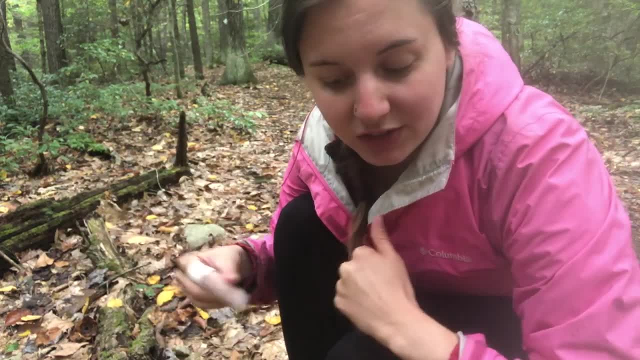 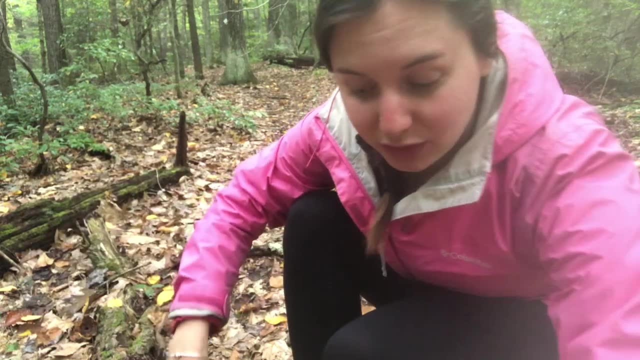 sure you're pulling up a log or a rock It towards you, up towards you, so that in case there's bees or something underneath it, it will go that way and not towards you. So if you were lifting it this way, you're trapping. whatever it is against you, you're lifting it towards. 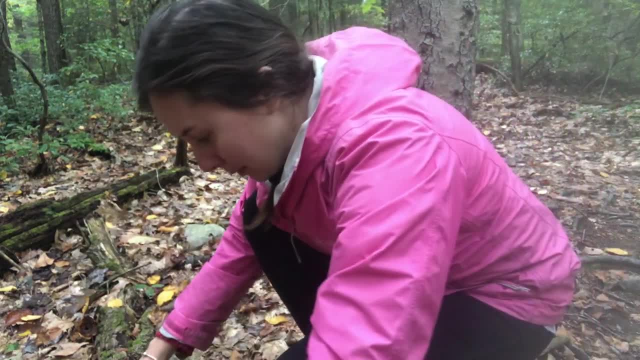 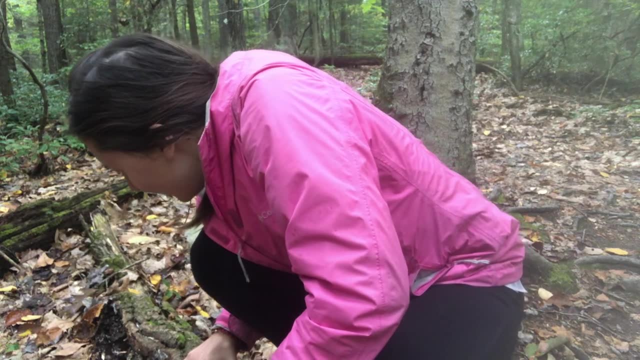 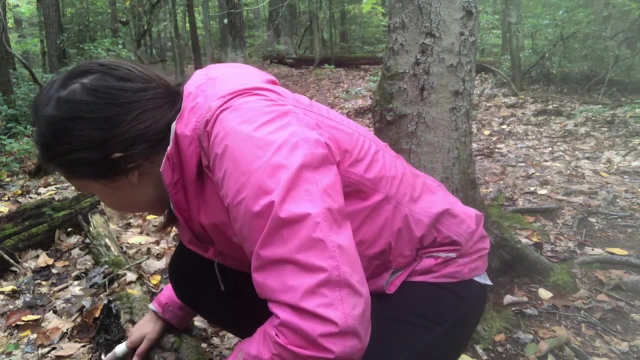 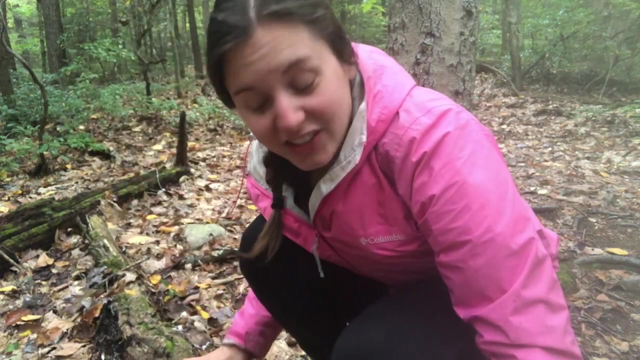 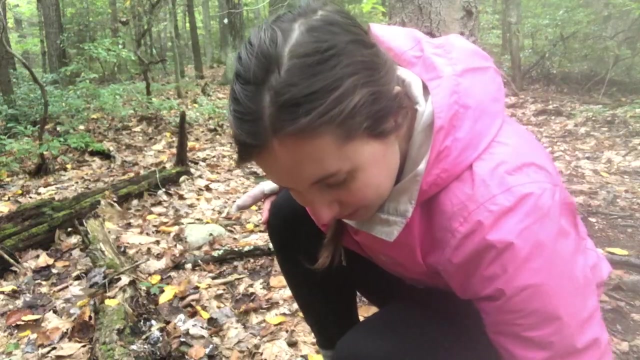 you. you have a barrier like a shield, So let's see what's underneath this one. There's actually nothing under this one. I wonder if it's getting too cold for salamanders. I hope we find one, Okay, so I just tried another log and I didn't. 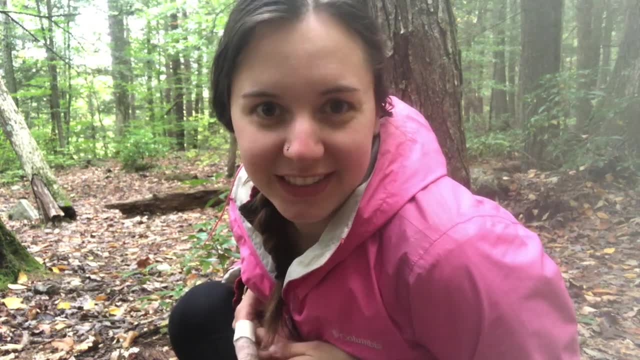 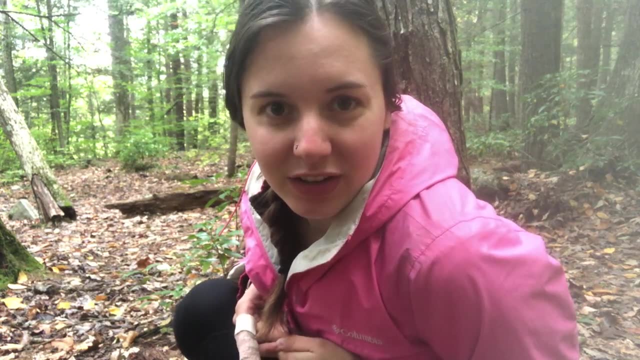 find any salamanders, but I did find one of my favorite organisms, A slug. So I believe this is a leopard slug, but it's a little more orange than I'm used to seeing. I'm going to show you what it looks like now, without disturbing it. 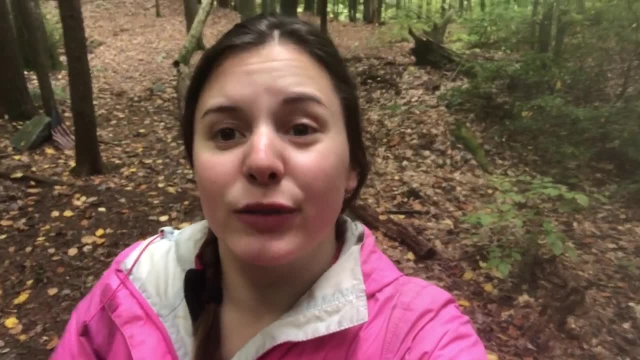 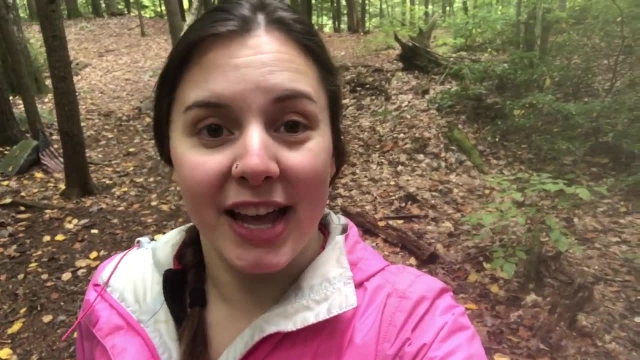 One important thing that I did not mention is, if you are turning over logs and rocks, you need to make sure you put them back the way you found them, because even if you didn't find anything, that log or rock could be a habitat for an animal or an organism that you didn't know. 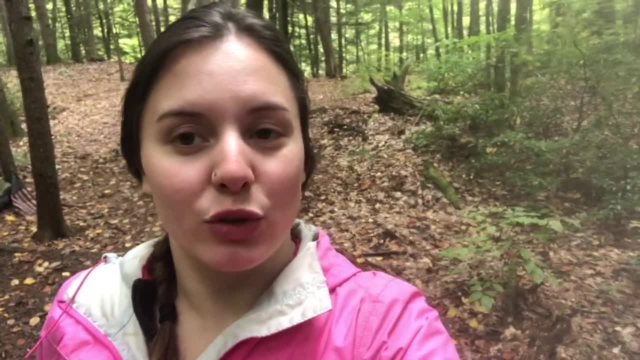 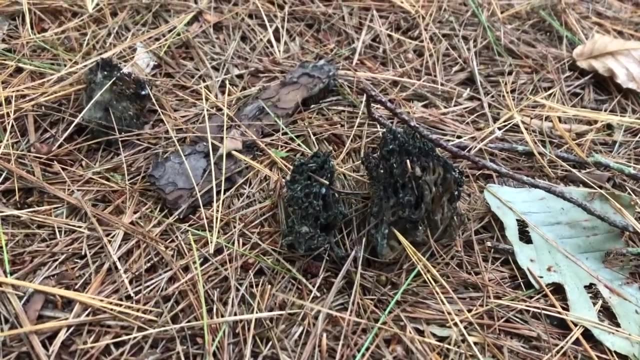 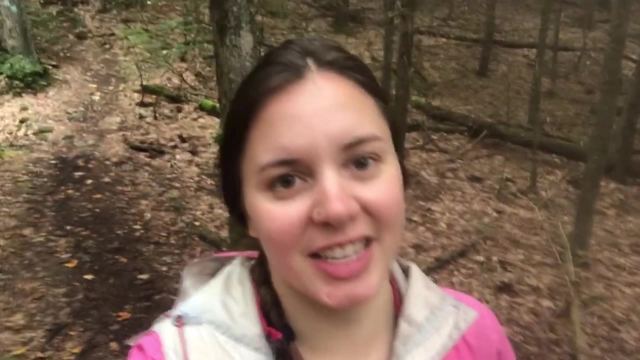 So make sure you return anything that you moved to its rightful place and you're practicing leave no trace. So unfortunately, today I have not found any amphibians, salamanders, toads, frogs, and I think it is because it's too cold right now, So they're all burying themselves under the 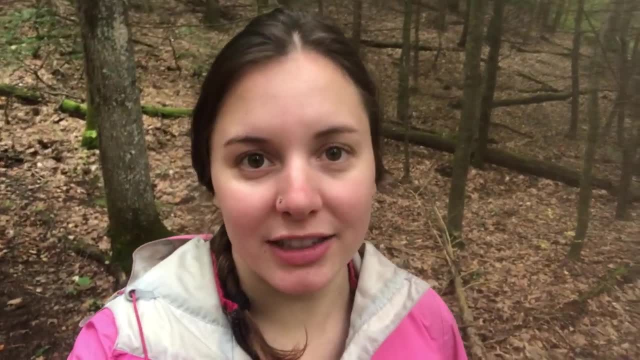 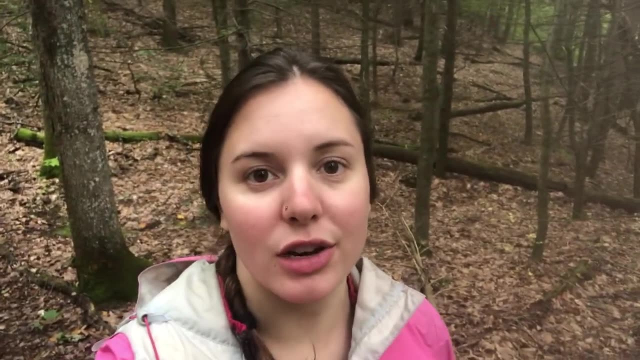 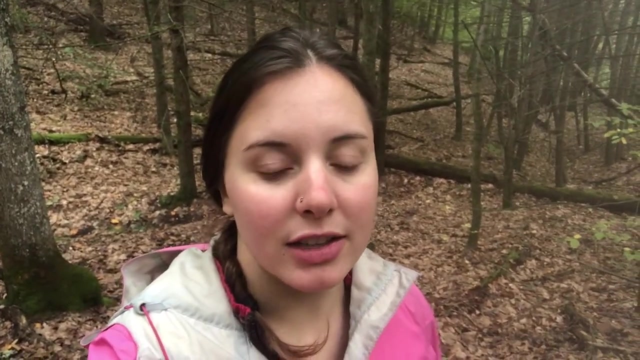 logs, rocks leaves to stay warm. But if you are in a warmer area and it's rainy out, I encourage you to go look for them so that, like I said, they like to be under logs, rocks leaves. It's the safest place for them and they are camouflaged there, away from predators. But I will insert some. 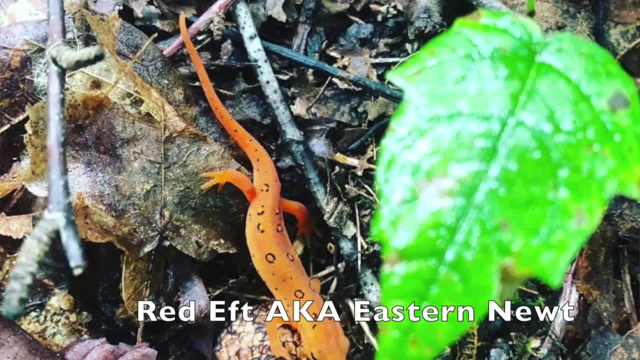 pictures of these in the video so that you can know what they look like. Salamanders are amazing creatures. If you're gonna pick one up or touch it in general, you need to make sure your hands are dirty. So right now, I'm going to show you how to do that. So I'm going to go ahead and 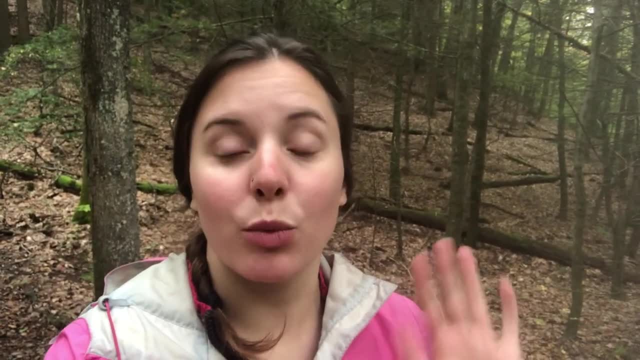 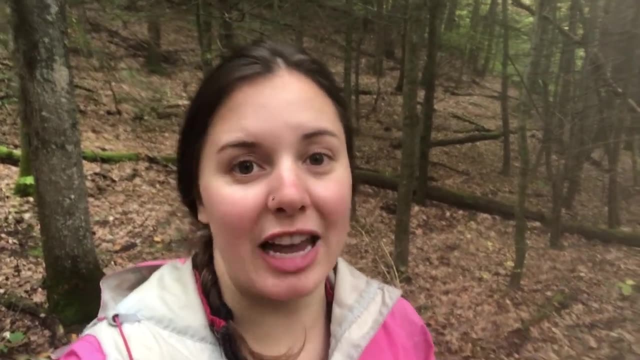 rub your hands in the dirt and make sure they're nice and dirty, because we have oils on our skin that actually clogs their pores and makes them unable to breathe, and sometimes it leaches chemicals and can hurt them or kill them. even So, if you are picking up a salamander, a frog- 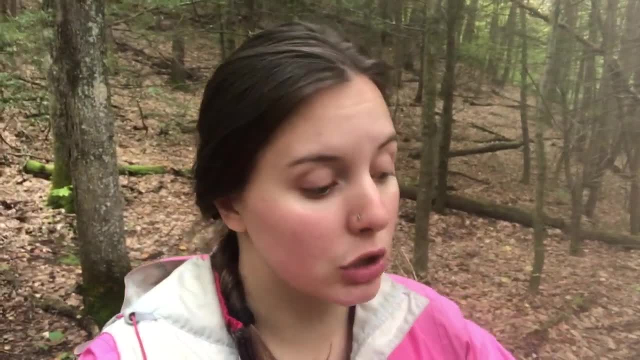 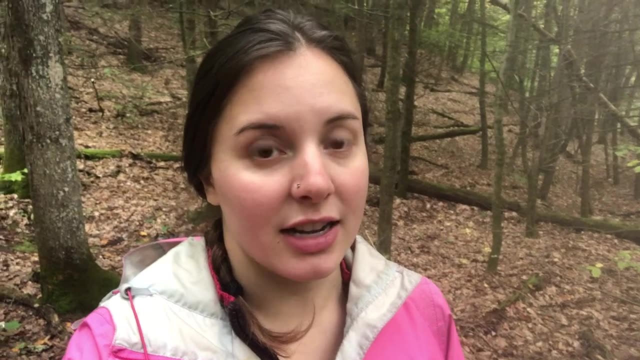 a toad. you need to make sure you have dirty hands, Like I'm talking. rub your hands in the dirt. Even better, scoop up some leaves so that they are not touching your skin. It's not anything that's going to harm you, but it's going to harm the organism, So you need to make sure you are keeping them safe. 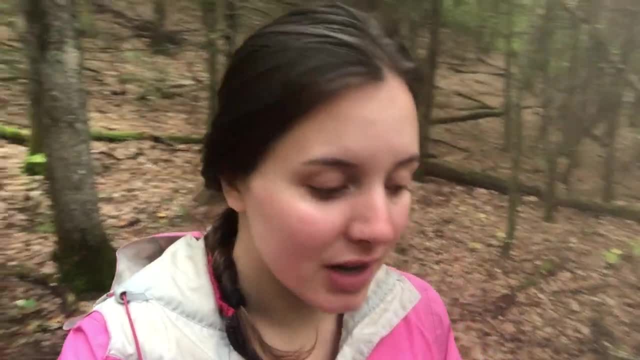 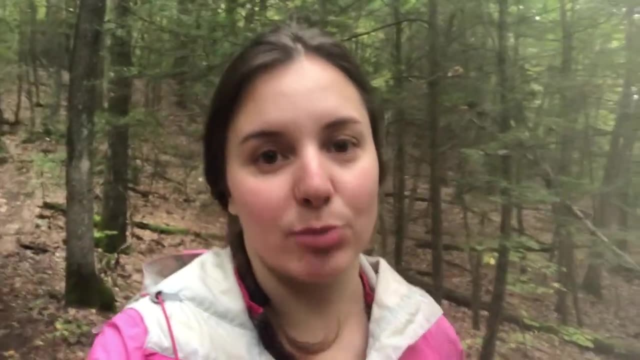 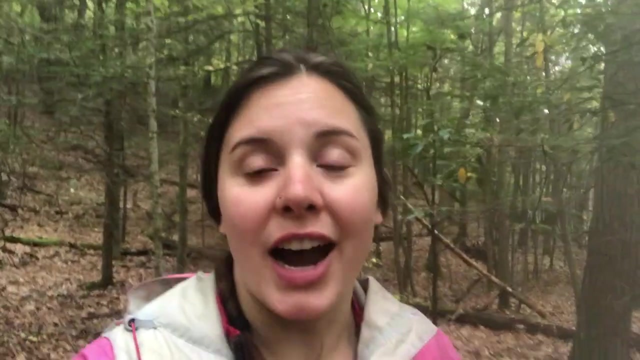 and you're leaving no trace because you are in their habitat in the woods. So I have a blog post that I wrote a while ago about how there's no such thing as bad weather. So if you want to learn more about activities you can do in the rain, in the snow, I encourage you to check out that blog post. 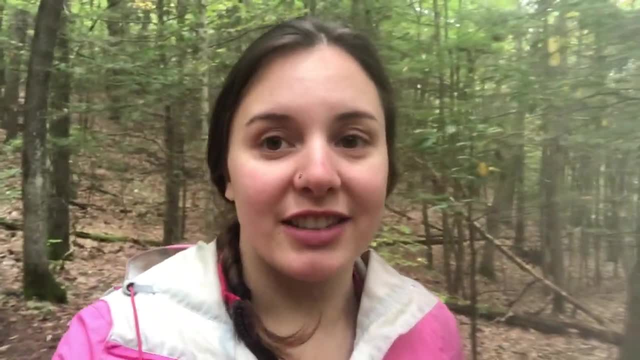 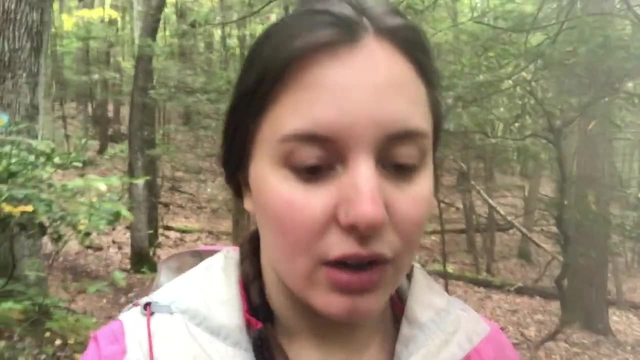 I will link it in the description below, because there's some great stuff and it goes into more detail about how to save your life. So I'll see you in the next video. Bye, pick up salamanders and amphibians. um, what else you can do in the rain? i just took this opportunity.